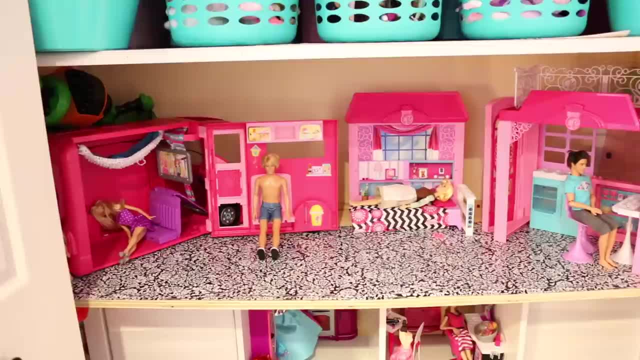 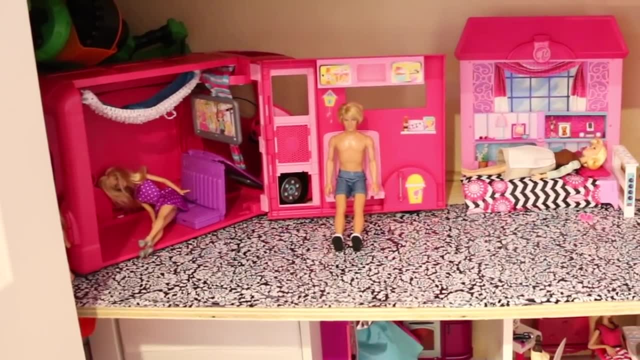 Another thing that we've practiced a lot is toy rotation. So this section of the closet here, this is Abby's side of the room, So this is her little toy table type area. We switch it out all the time, So right now it's Barbie's, Sometimes it's Lego land, we call it. We put all the Lego. 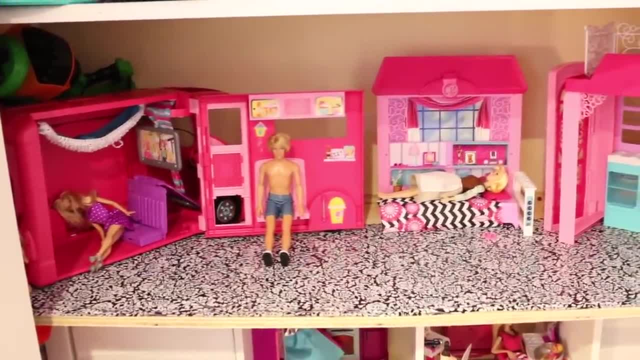 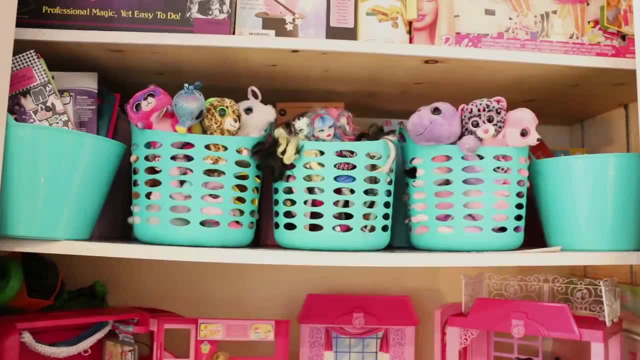 on here. Sometimes we switch it out with princesses. It's constantly changing and I find that the stuff that's you know, set up is the things that they play with the most. So I really do a lot of toy rotation. Also, for toy rotation we have bins in behind other bins and they get 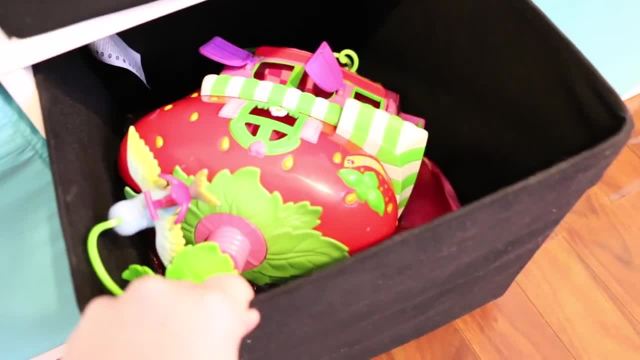 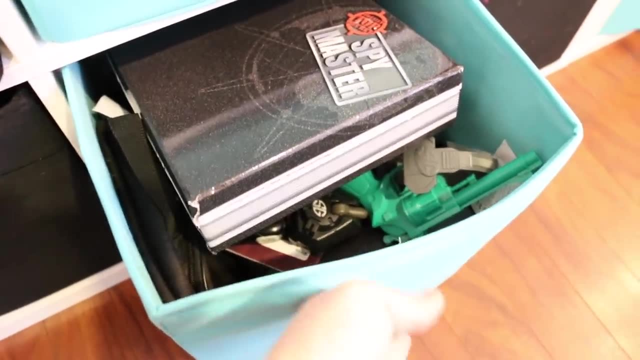 rotated, pulled up to the front and also rotated in other areas of their rooms. So the ones that are, you know they're not able to access those. those are harder to get to, They don't play with as often, but when we bring them out and switch them to other areas of the room, then they start. 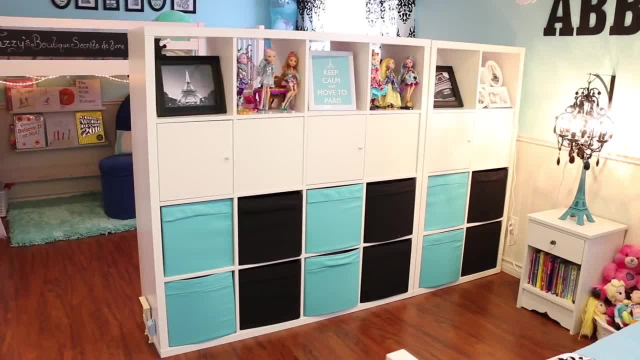 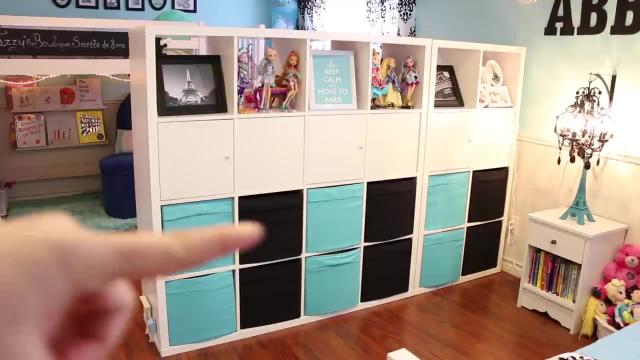 playing with those ones more often and we pack away the other toys. Instead of dressers, we use this wall divider. It's just Ikea shelving and bins and clothing goes on these bins. here. All of these are filled with different clothing, and then down here these are toy bins that the kids use on a 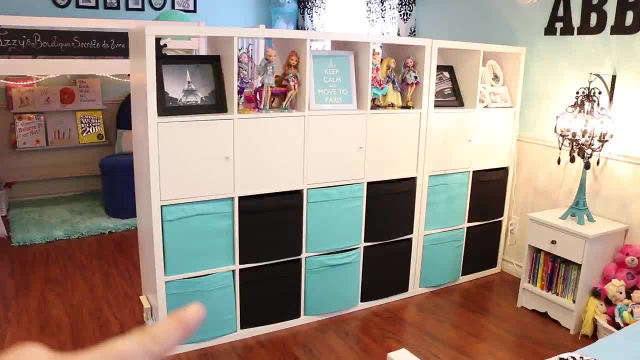 regular basis. They don't have to be in the closet. They don't have to be in the closet. They don't have to be in the closet. They have a lot of toys, I know, but we rotate the things out of here into. 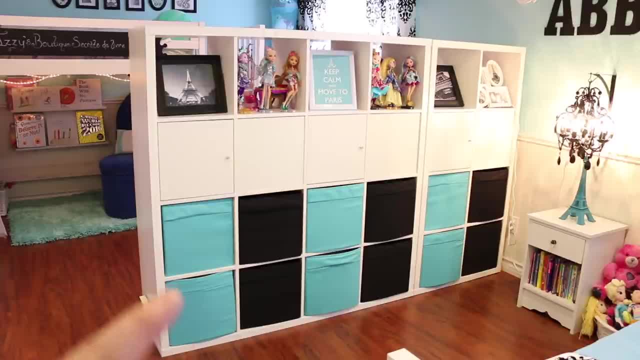 the bins in the closet. These are the ones that they generally play with the most, but we're constantly rotating them out. That way, they have new and fresh toys to play with, And all they do is pull out one of these bins and they have a complete toy set in the bins at the bottom there. 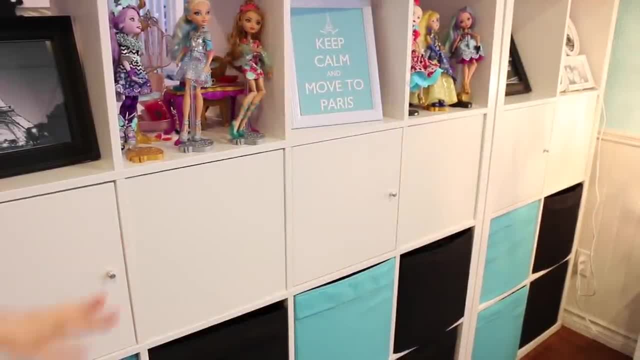 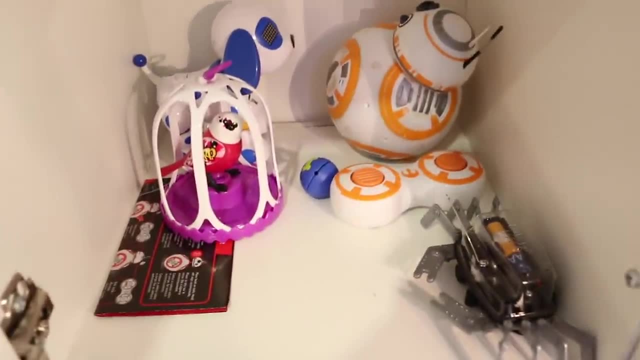 Another thing we do that I think is really key in keeping kids organized and their room clean is giving them little hidey spots for all of their stuff. So we have different cubbies and baskets hidden all over the place where they're encouraged to put their treasures. 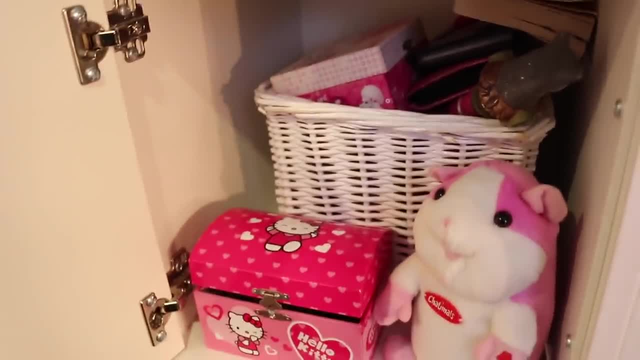 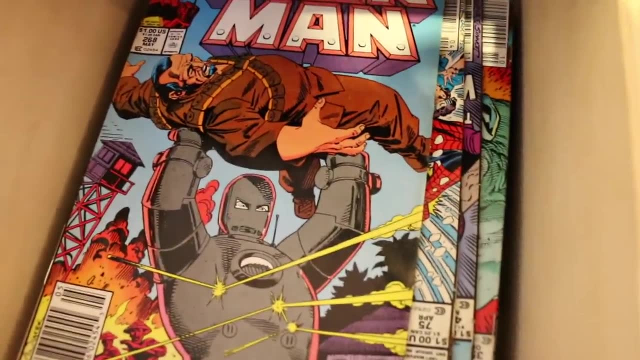 Kids are like mini hoarders and they're constantly collecting things that are so important, whether it's drawings that they do. Even McDonald's toys at the time are so important. but you need a place to put those things, So a designated bin or basket, or a few little baskets. 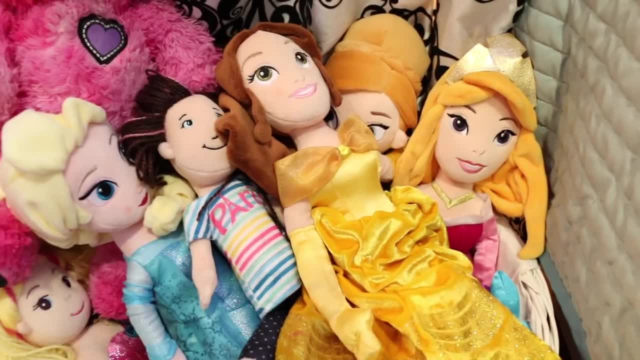 for all of their special treasures are a way of really keeping that stuff contained, and then you just help them go through it every couple of weeks. So it's a really cool way to keep your kids organized and organized so that they don't have to wait a couple of months to purge it down when 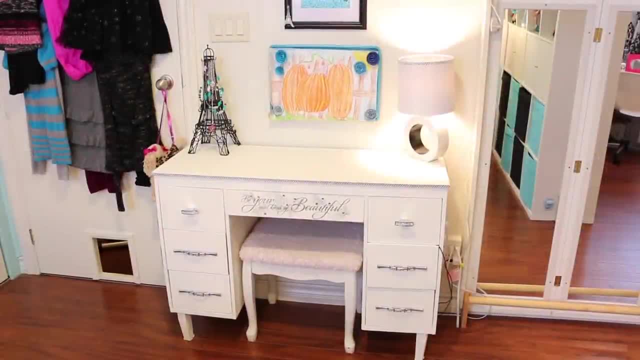 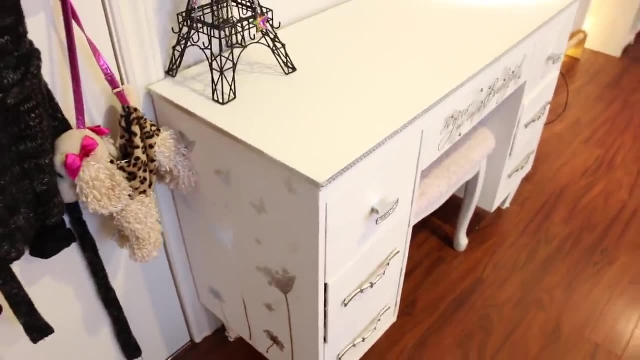 it gets out of control. Another thing we do to make sure that they're really going to stay, you know, organized when it comes to homework and that type of thing, is create them a little section where they can be productive, So have it all at their fingertips so they're not looking. 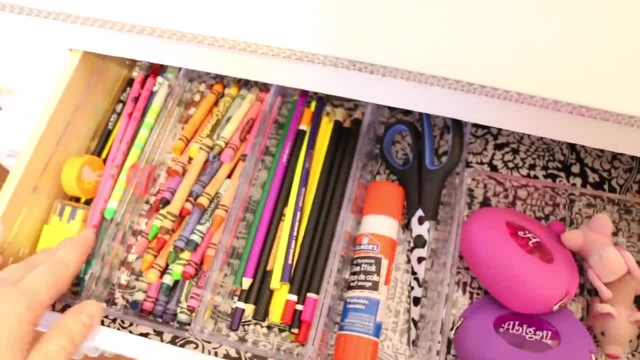 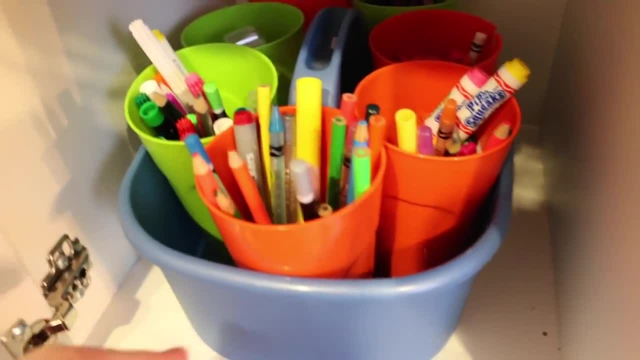 for things like pens and pencils, when it comes to homework or pads of paper, All of the art supplies, whatever it is that they love to use, having a designated spot for it. Even if you have a small space you can create like a little space for them to put their treasures. So if you have a small 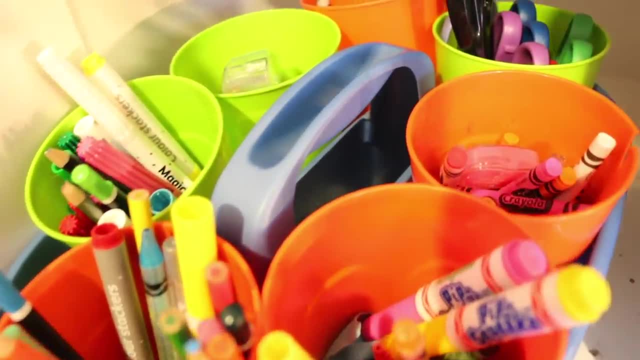 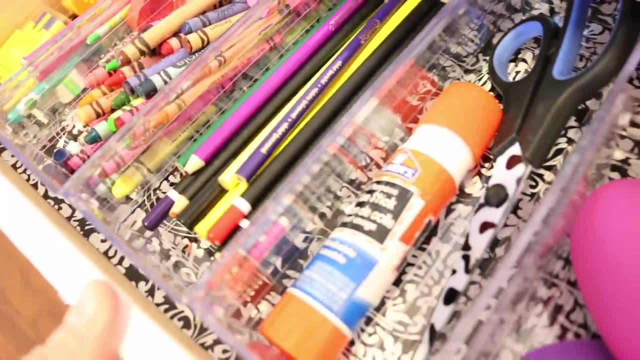 portable homework station, something that just has, you know, all of the things they need to complete homework on a regular basis: pencil crayons, maybe. crayons, markers, rulers, calculators- all in a really convenient spot so they're not wasting time looking and trying to find the things. 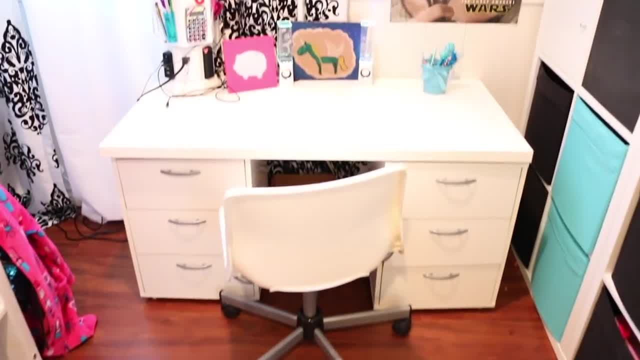 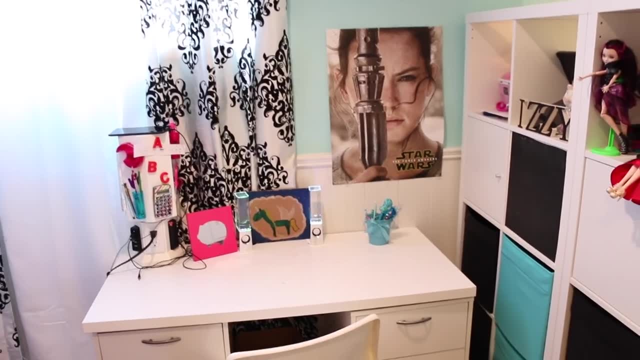 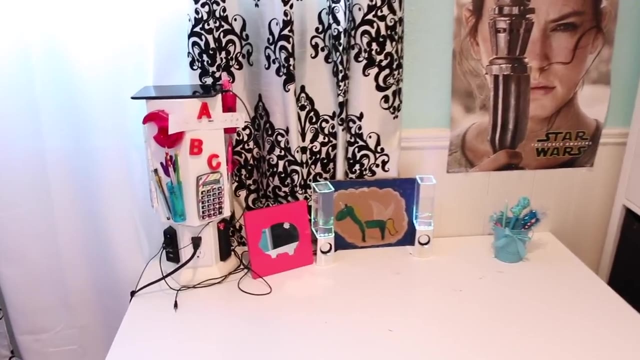 they need to be productive. Here's Izzy's desk on her side, and she's got a spot for pens and pencils that she uses for her homework too. She's a big Star Wars fan, so that's her Star Wars poster, But, as you can see, she has her calculator. she's got her tape, everything right there- her charging. 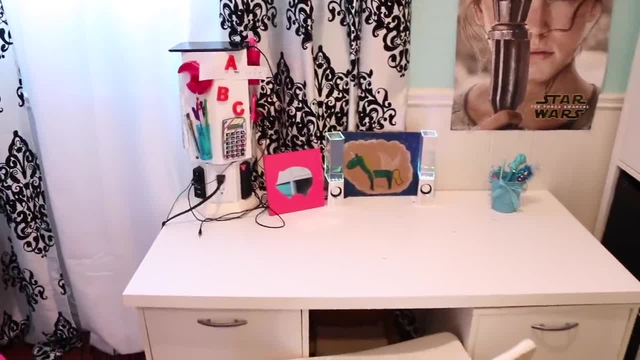 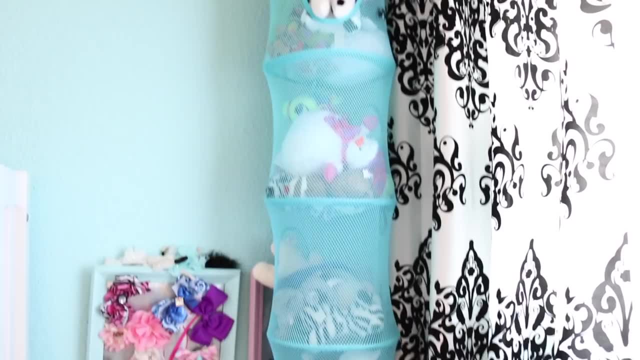 station for her iPad. everything right there at her fingertips, where she can be really productive without having to look for things. I love these hanging organizers for stuffed animals. They hold so much and they're about five dollars from Ikea. You could find them at other big box stores too. 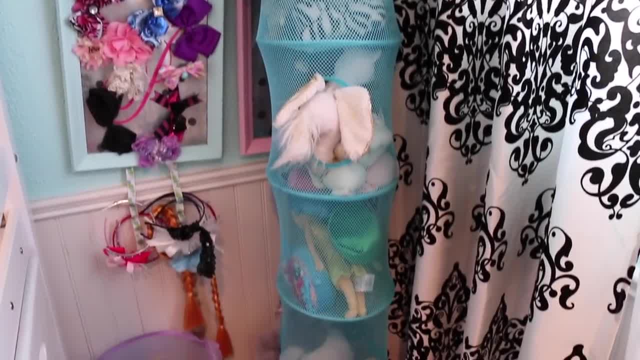 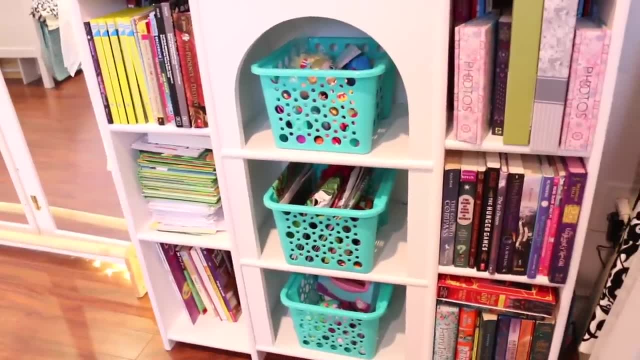 but the cheapest. I've found them with the most color selection is definitely Ikea. Some fun ways to organize books besides just traditional bookshelves. There's these little- I don't know, they're shelves with a lip on them. These came from Ikea as well and they're great for displaying the most favorite books and getting 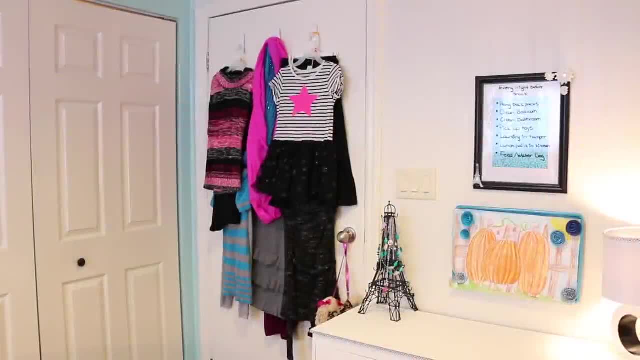 them, you know, up off the floor, Just so. clothes aren't everywhere, especially clean clothes. what we do every week is we hang different outfits, just random outfits, on the back of the door. It already has the shirt, the pants, the sweater, whatever they need to complete an outfit. 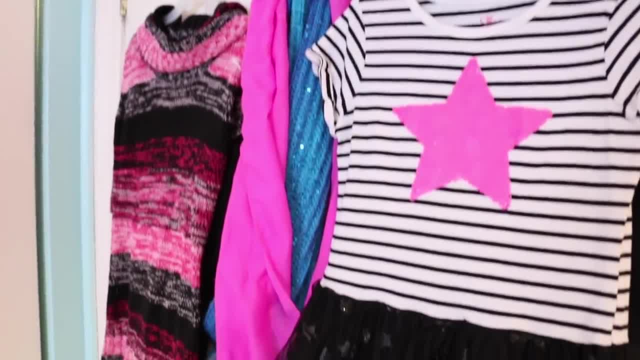 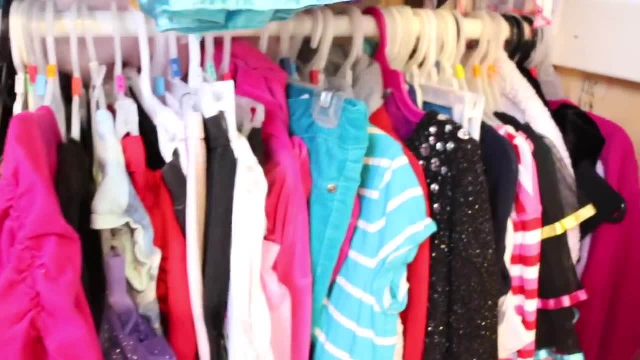 all together and they can just grab it off the back of the door and get dressed. So they're not, you know, going through their closets and going through their- you know- dresser bins trying to find outfits. when it's rushed during the morning, Everything's already set out for them and ready to. 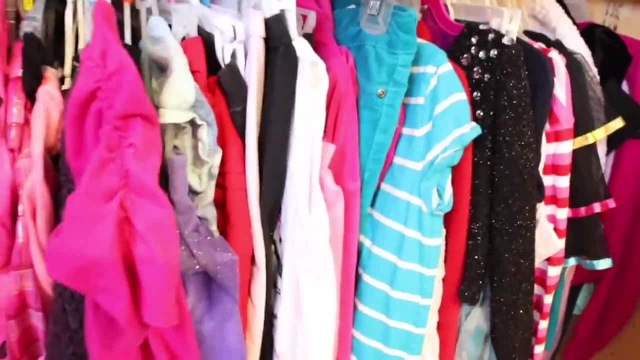 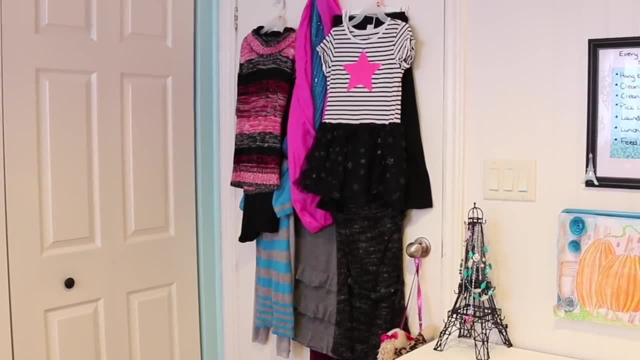 go. I really recommend, if you have kids who are constantly putting clean clothes all over the floor trying to get ready in the morning, that you set aside some outfits already prepared for them, just to make life a little easier. I don't pick what they're going to wear and they can. 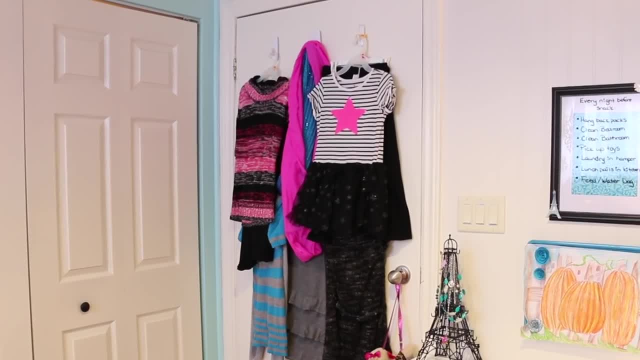 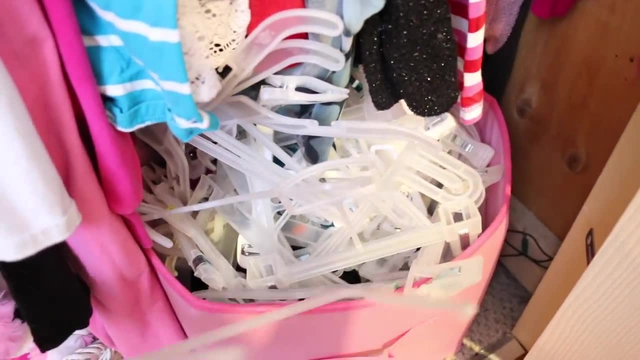 definitely still choose from their closet, but this just gives them, saves them, a little bit of time every morning. On the bottom of their closet, we actually have a hanger bin, and this is a spot when they are, you know, taking off clothes, to put it, Instead of leaving the hangers all over the floor. 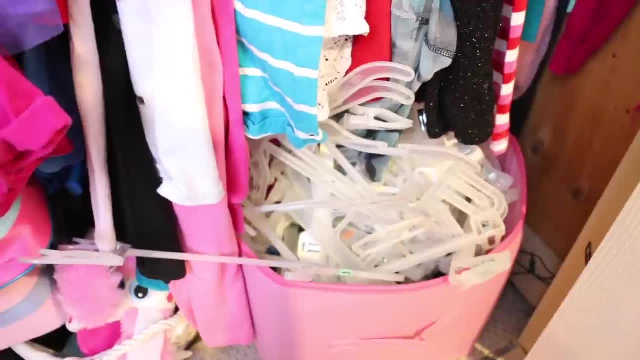 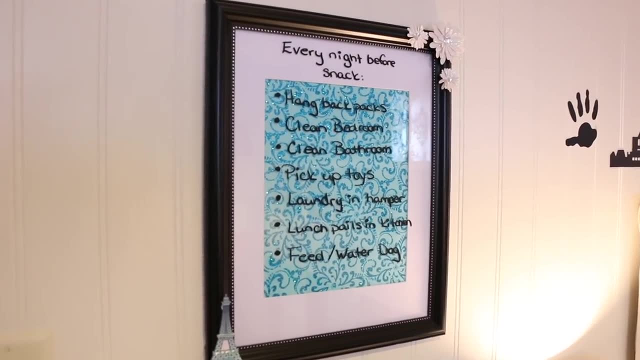 they've got a spot where they can just toss them in, and then, when we're putting away laundry, all we have to do is put the hanger bin on the bed, and it's easier to put away clothes. A chore chart is a super great way of just letting them know what you expect from them every day. 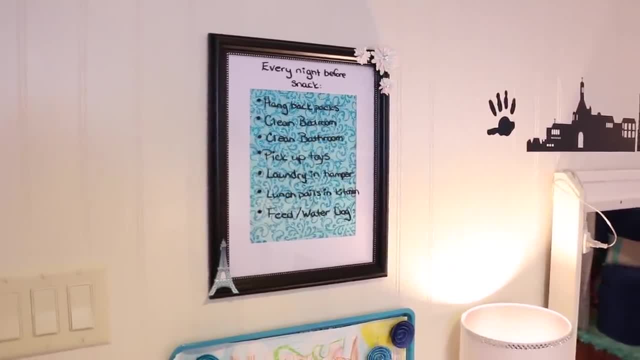 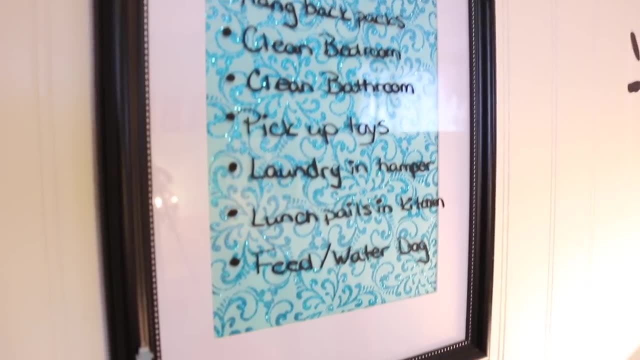 and I love having it posted in their room all the time. This is just a picture frame with dry erase marker on it. They know what they have to do when they get home and all the things they have to do before they're allowed a bedtime snack every night. Just take a look around your kid's room and see where. 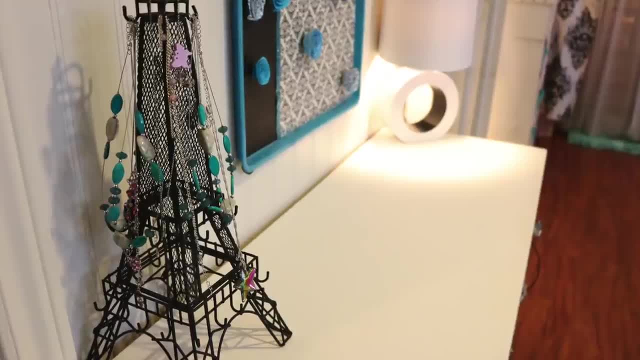 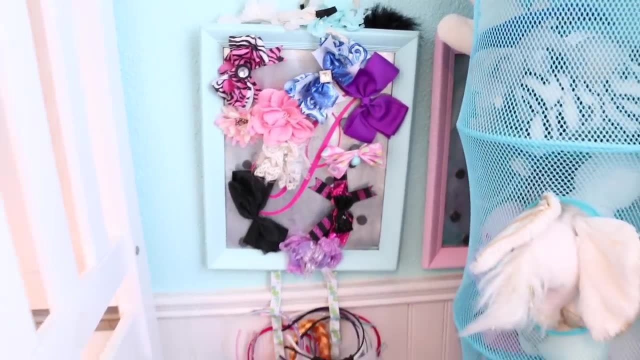 their clutter spots are: If you've got a lot of artwork and papers all over, why not make them a little bulletin board where they can display it? or if you have hair bows and jewelry, why not get them some sort of holder to contain and organize those? Once you've set up systems for kids and you show. 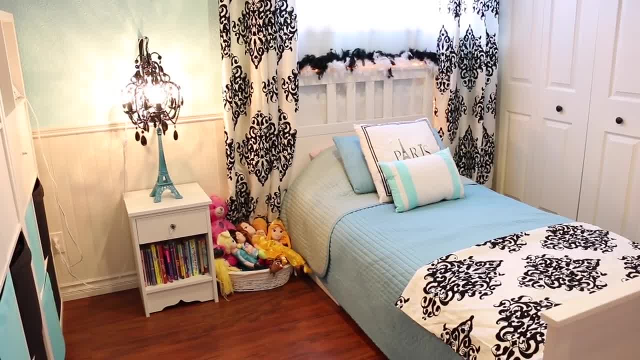 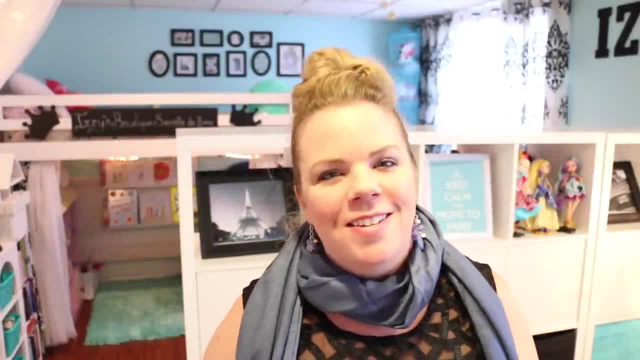 them how to use it. it's pretty easy for them to follow along and keep their room really organized. So thanks so much for watching. Set your kids up some really easy organizing solutions today with sorted bins. Think about doing some toy rotation and perhaps separating some clothes. 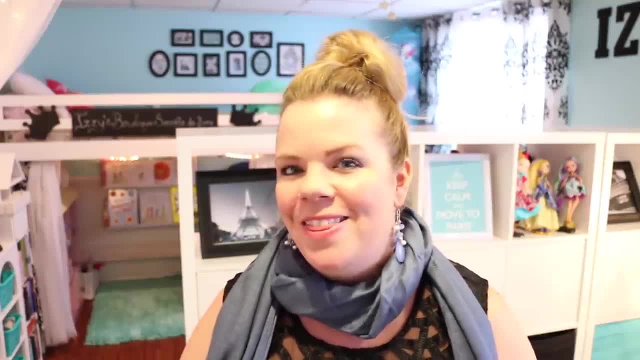 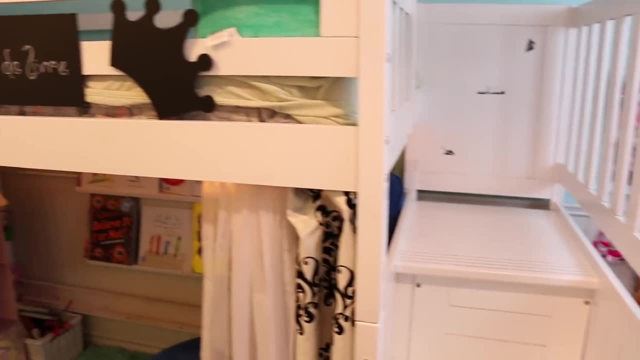 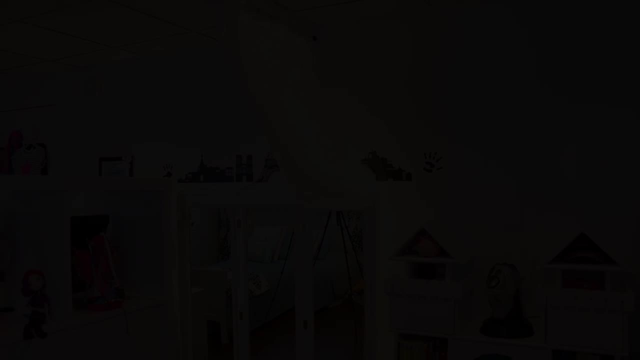 for the week to make keeping their room a lot easier. Thanks so much and we'll see you next time. Thanks so much for watching. If you want to see this whole Izzy and Abby room tour, you can click here for a room tour video. and also make sure you subscribe, because on Monday, February 29th, 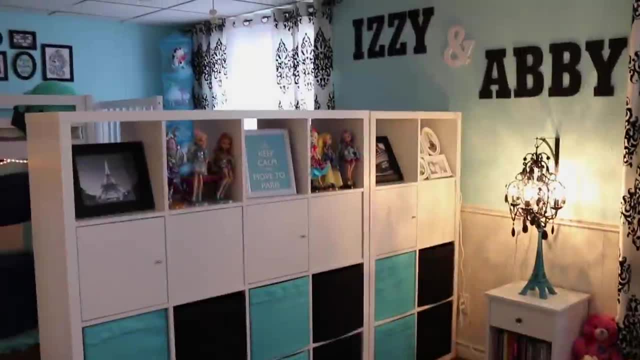 we're doing a giveaway for a brand new Roomba valued over a thousand dollars. All you have to do to enter is be a subscriber. So thanks, and we'll see you next time.